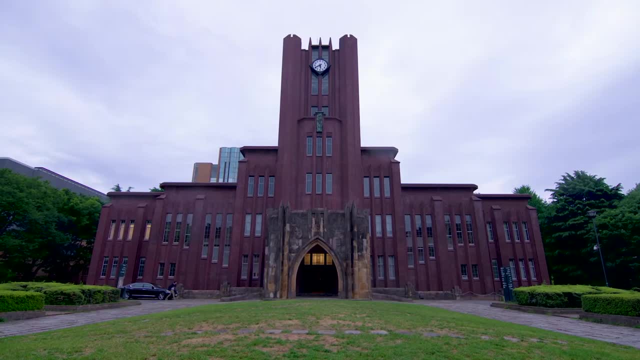 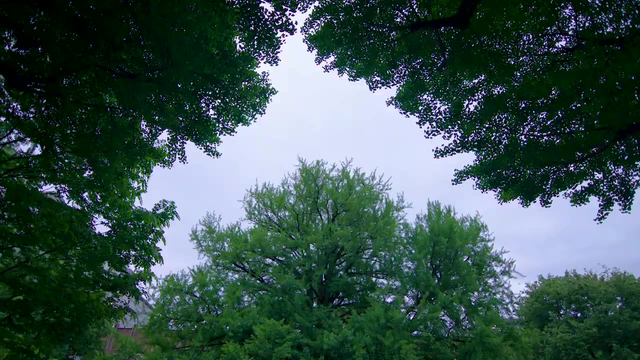 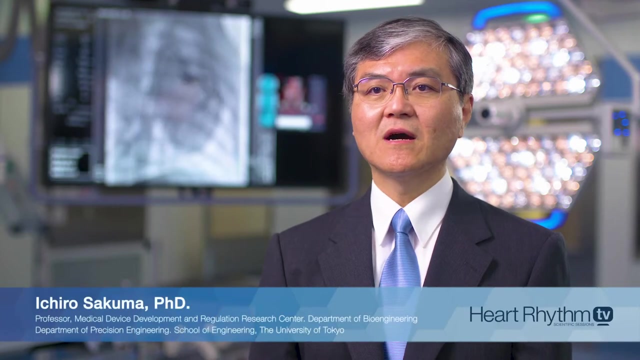 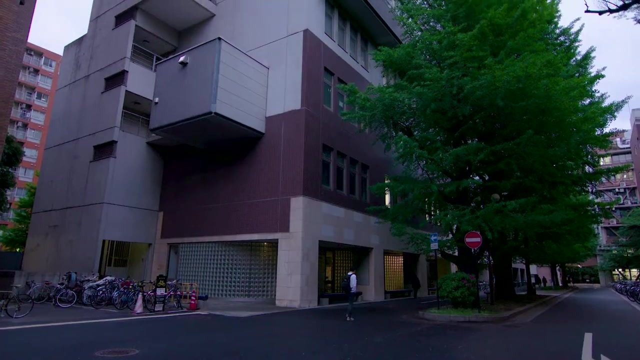 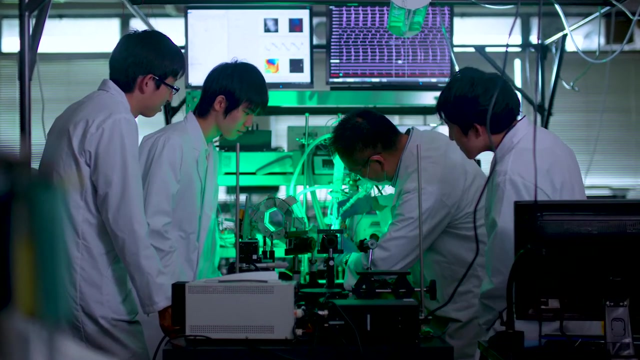 The University of Tokyo is the oldest and top university in Japan, having the world's oldest Faculty of Engineering. In Faculty of Engineering, biomedical research has been conducted since the 1950s. Biomedical Production Engineering Laboratory was established in 1981 as the first laboratory purely dedicated to biomedical research in the Faculty of Engineering. 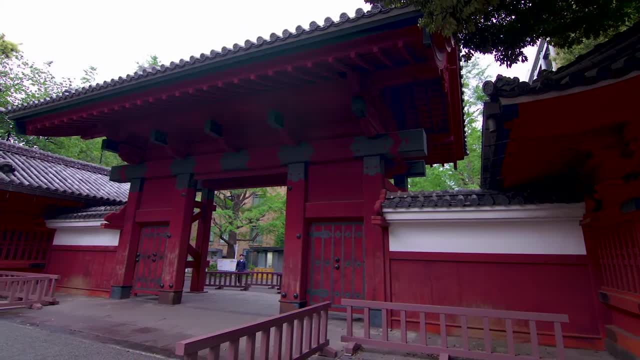 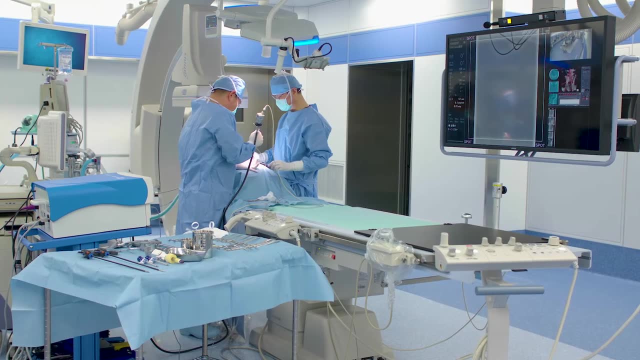 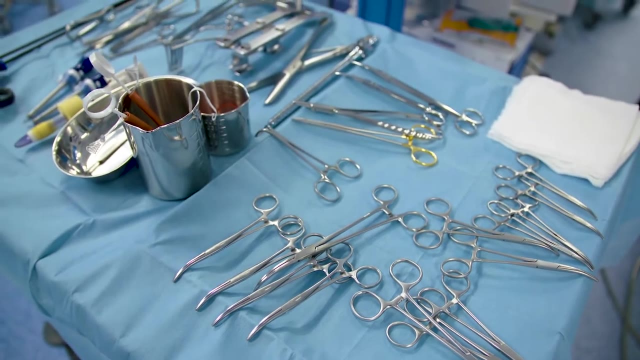 Department of Bioengineering has started its graduate program in 2006.. Medical Device Development and Regulation Research Center was opened in 2012 for promotion of translation research and regulatory science for medical devices. Various bioengineering research is now conducted in the Faculty of Engineering. 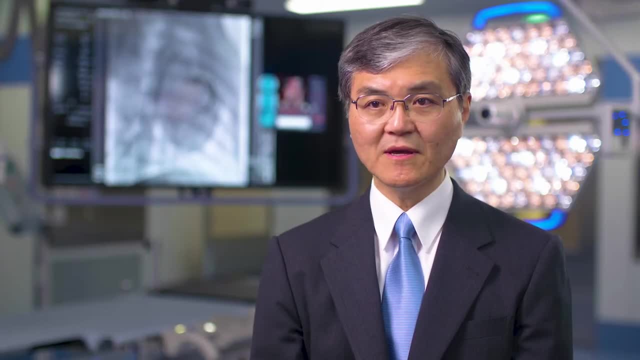 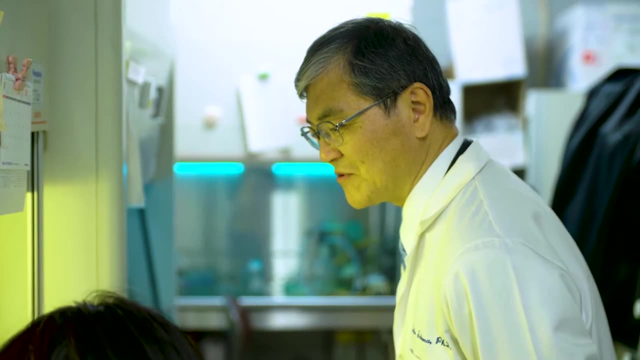 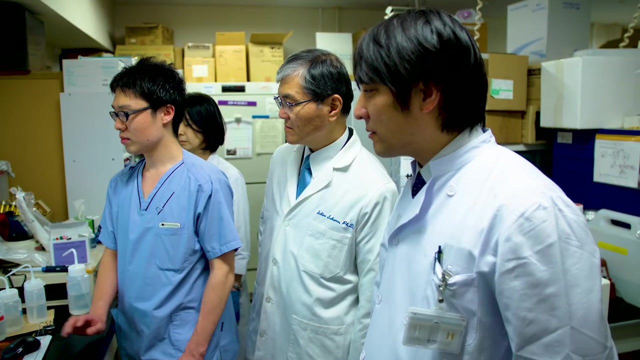 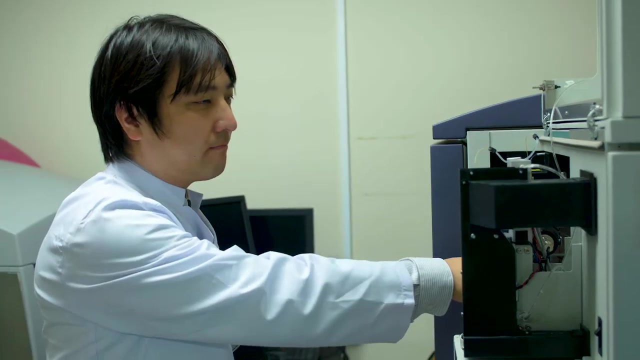 In collaboration with Faculty of Medicine and the University of Tokyo Hospital, Biomedical engineering research in arrhythmia are also very active in this university. In our laboratory we are focusing on the development of technique to visualize the arrhythmia events that is indispensable for analyze the mechanism of initiation, maintenance and termination. 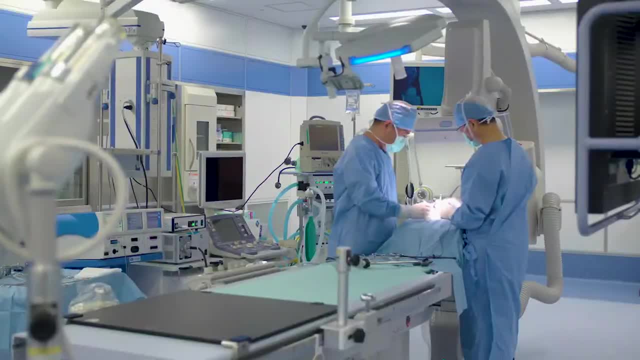 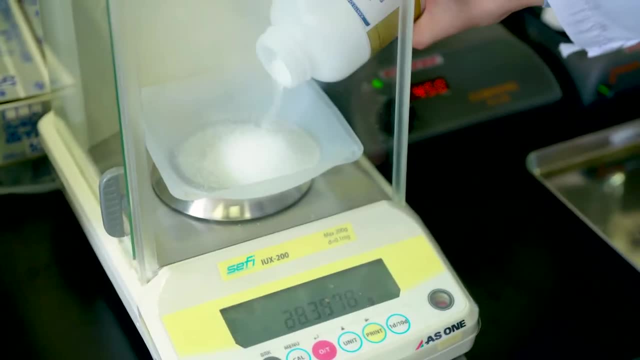 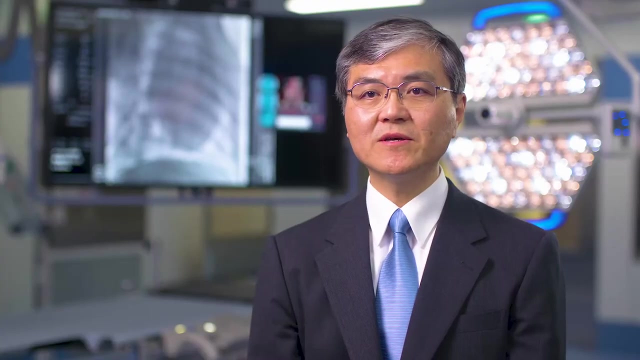 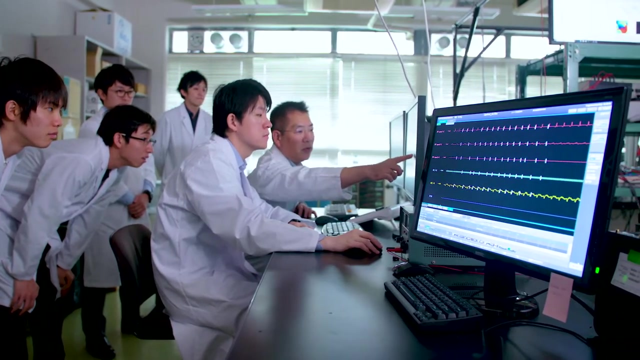 We have developed an optical mapping technique. This technique is based on various cognitive action potential, with superior signal to noise ratio and high spatial temporal resolution. We also conducted some signal processing. obtained data. We recently proposed some new imaging processing method to analyzing dynamics of arrhythmia. Computer simulation is also used to discussing the experimental results Through 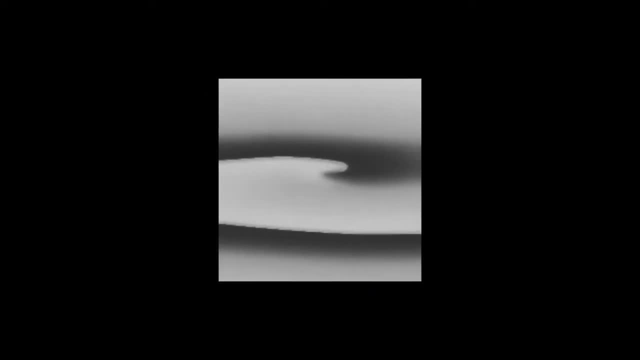 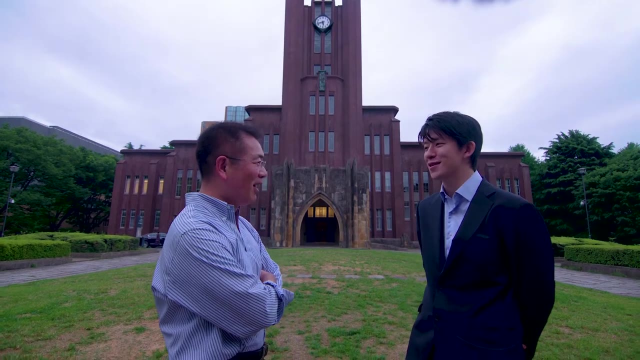 these studies we are studying an optimization of the electrical signal and the signal resolution stimulation or other physical stimulation for the termination of Alzheimer's. Other than these activities in University of Tokyo there are many studies, including molecular science study and also the computer science study. 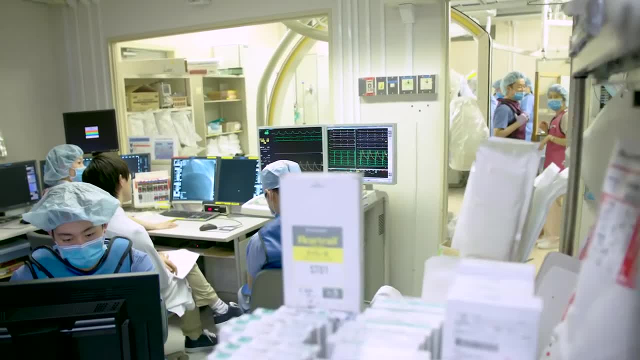 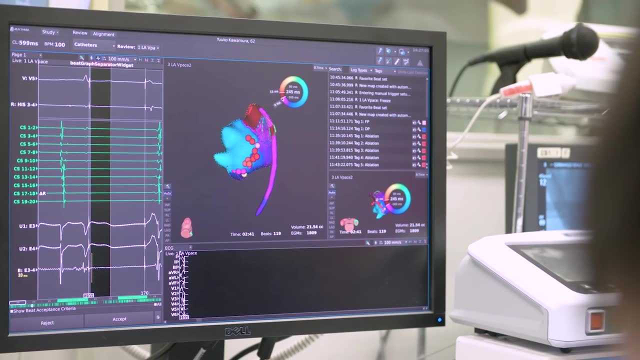 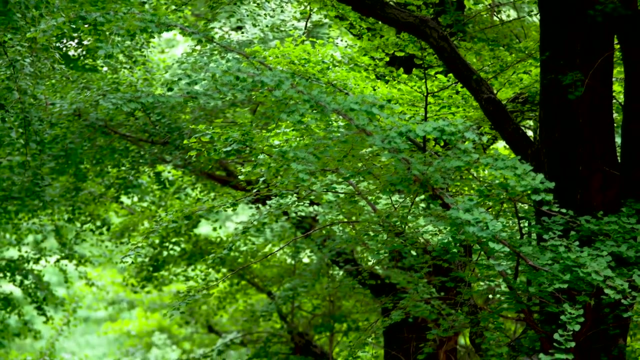 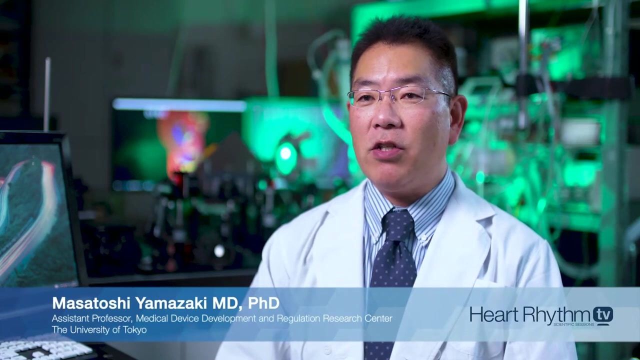 One of the results is that highly complex, multi-scale, multi-physics computer simulation of cardiac events that is widely used in the US clinical studies. Despite of many years of research, the precise cardiac fibrillation mechanism of the underlying initiation and maintenance are poorly understood. 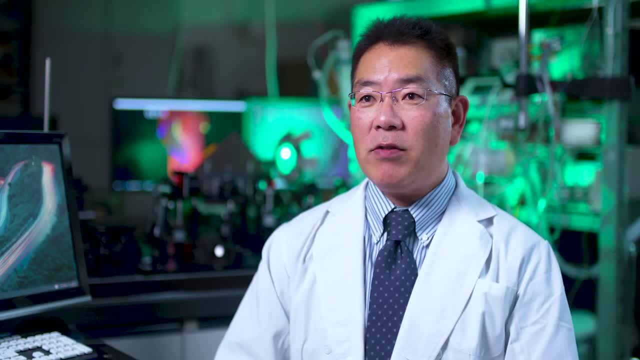 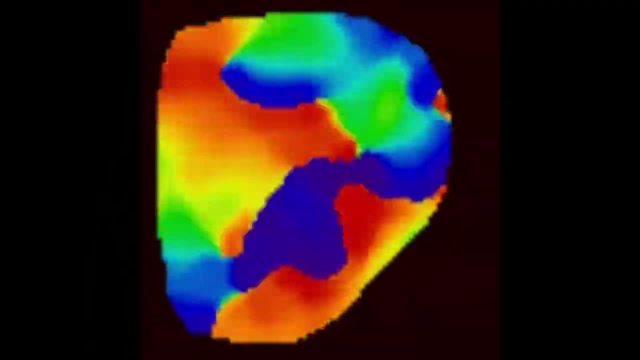 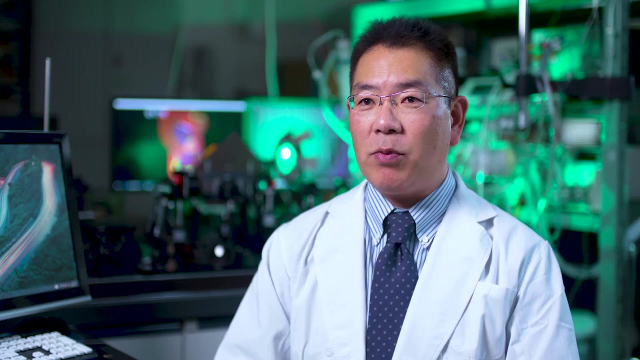 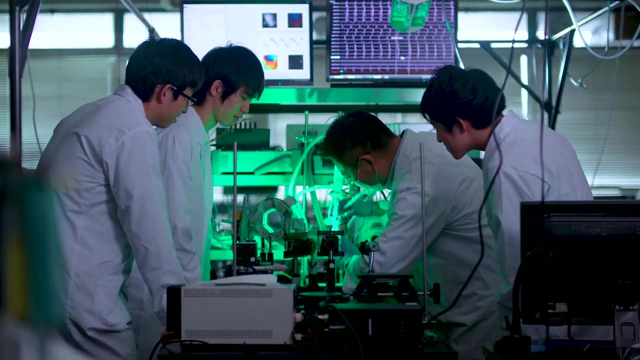 Since about 100 years ago, many theoretical and experimental studies have suggested that spiral wave re-entry, also known as rota, rotating around a functional obstacle like a hurricane and tornado, is a major mechanism of cardiac fibrillation. While the detections of rota in the clinical setting is carried out with the use of 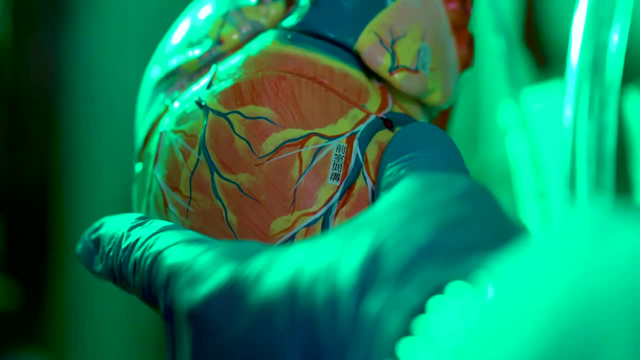 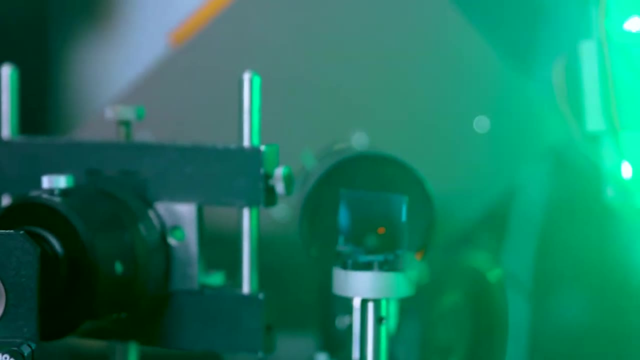 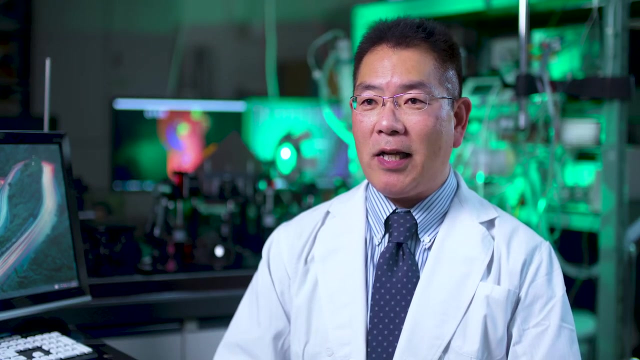 multiple electrode mapping system or body surface mapping system. those are still challenging on account of a relatively low spatial resolution mapping system. Our objectives are, first, to explore spiral wave dynamics, specifically in cardiac fibrillation, using high-resolution optical mapping system and computer simulation. And thirdly, 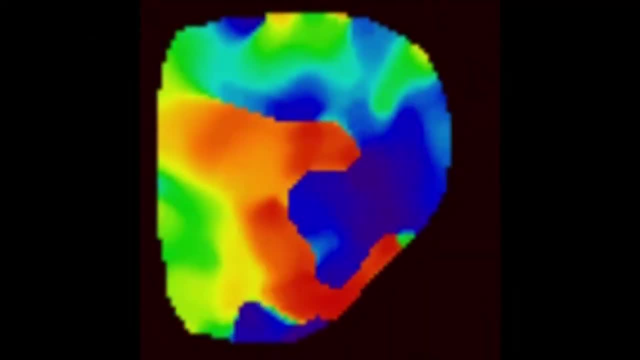 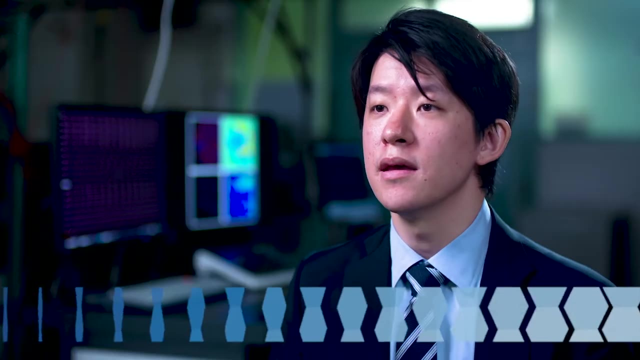 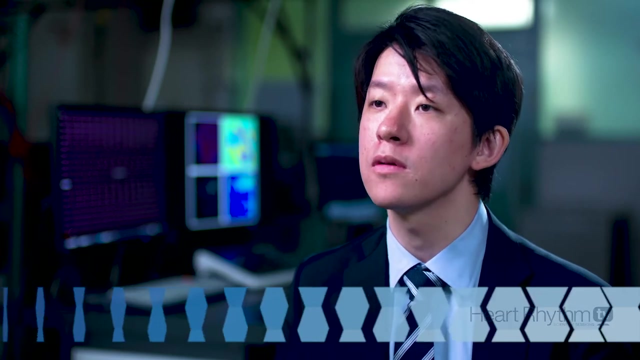 to examine how radio frequency ablation of spiral wave effectively terminates and prevents cardiac fibrillation. The interest of our research is how to control spiral waves during arrhythmia. To explore the way of control, optical measurement systems and computer simulation models have been used. 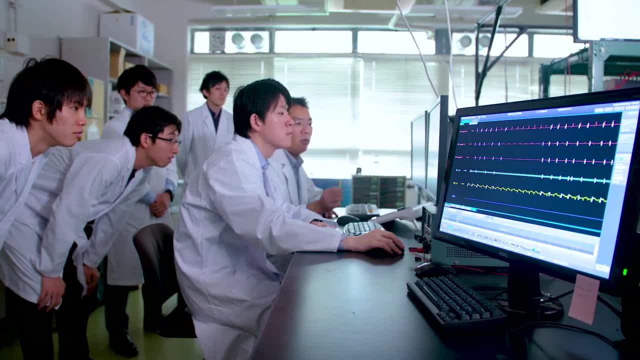 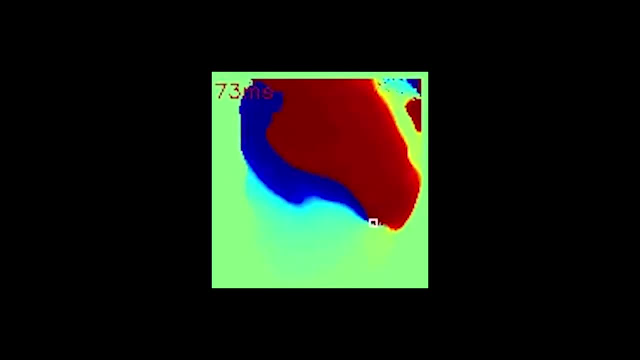 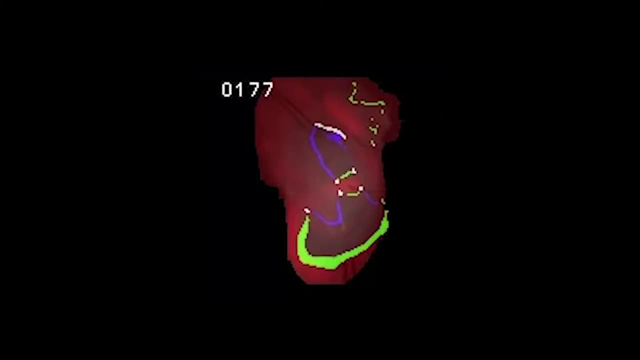 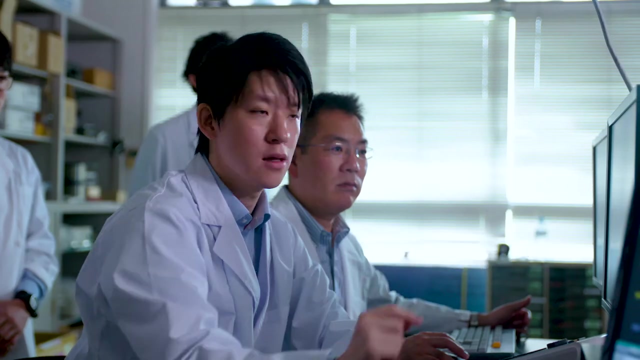 On the other hand, for better understanding of these results, an objective analysis method for chain probability is needed in order to quieresize a greater range of ranges of Ung Safark along the outlook ofikum's oscillating rehabilitation data for meaningful spiral waves: plantensemble analysis. 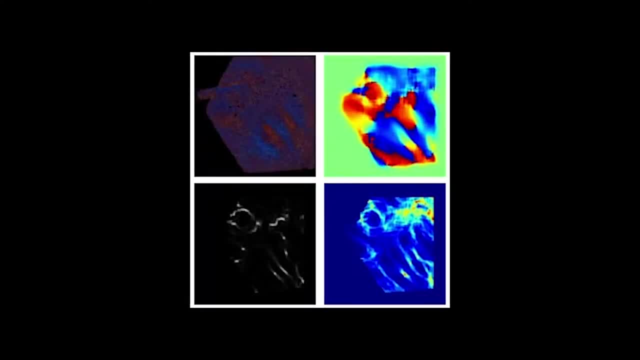 And the lack of a complicated activation pattern is necessary. That's why we have invented a quantitative analysis method of spiral waves trajectories. The method named phase-variance analysis allows us to identify the interaction process of multiple spiral waves. By using this method, we can evaluate the effect of electric stimulations and clarify 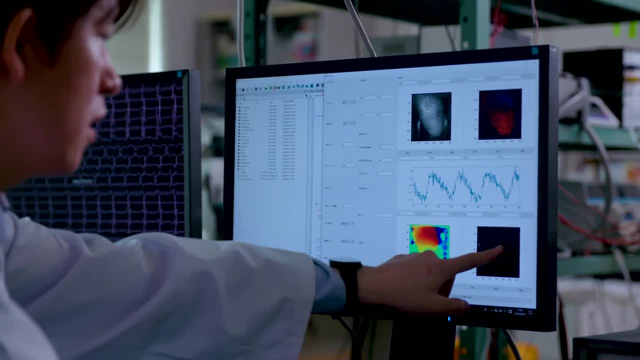 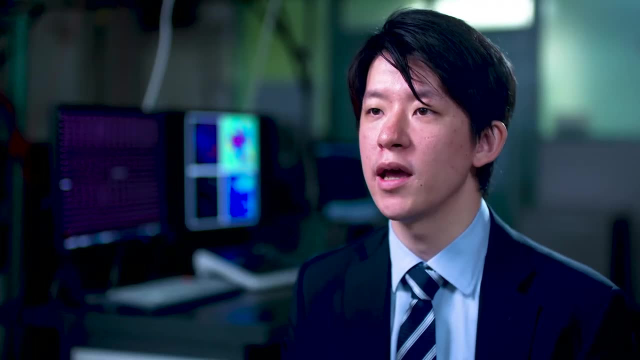 the mechanisms. The same method is also useful to analyze- So it is a matter of course- complicated activation pattern during fibrillation. Based on the knowledge of these basic researches, we are challenging to realize more reliable and effective treatment of arrhythmia. 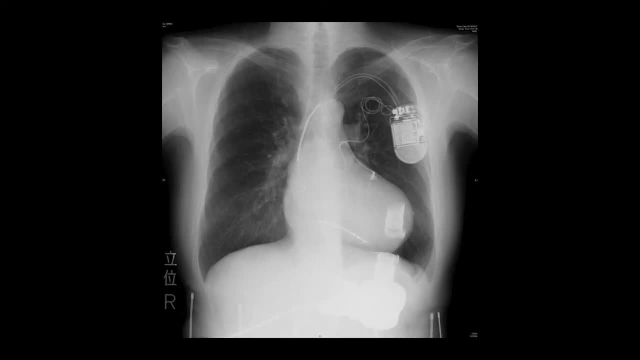 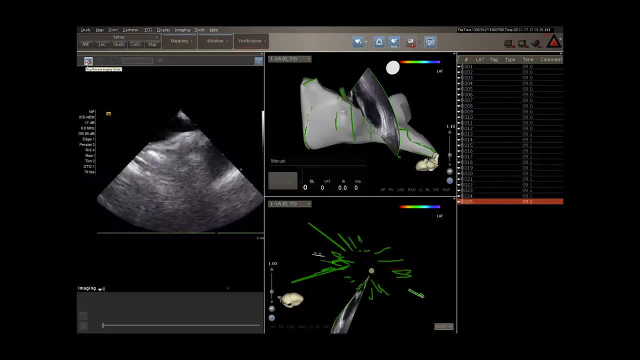 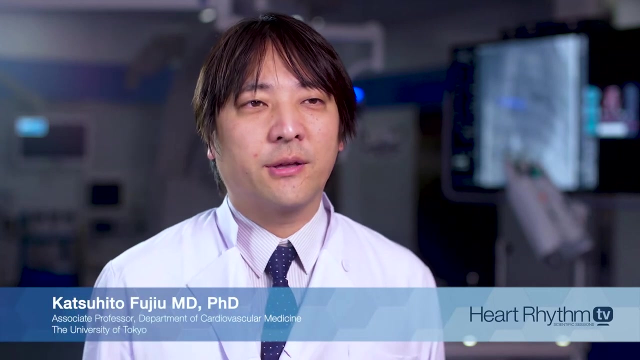 The University of Tokyo Hospital can handle all of arrhythmia from pediatric to aged patients by ablation and all kinds of devices. In the basic research we are trying to find the new molecular mechanisms, how severe heart failure and refractory arrhythmia develop.